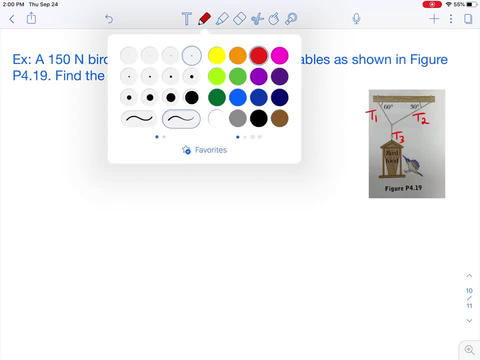 is to solve for each of those cables, And what I'm going to do is I'm going to kind of transpose those cables and those angles onto an XY coordinate, because I think that's going to help us kind of visualize those forces a little bit better. And so we basically have one downward 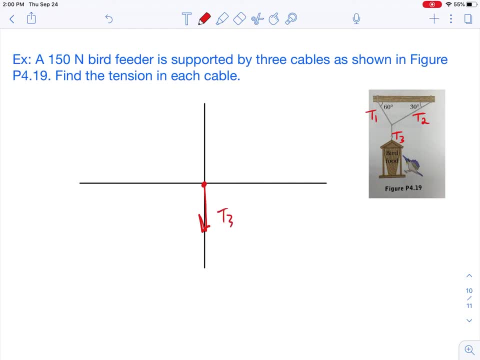 force is T3. And, based on the problem, we know that that is a 150 Newton bird feeder. So I know that T3 equals 150 Newtons and would technically negative because it's going in the downward direction. Now I'm going to draw my T1 and T2 forces. 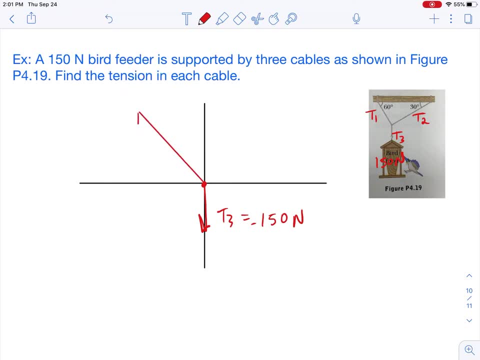 Like such all right, where this is going to be a 60 degree angle And this is going to be a 30 degree angle, And that just goes back to alternate interior angles, right? So the 60 is up here and the 30 is up here in the problem because they're alternating. 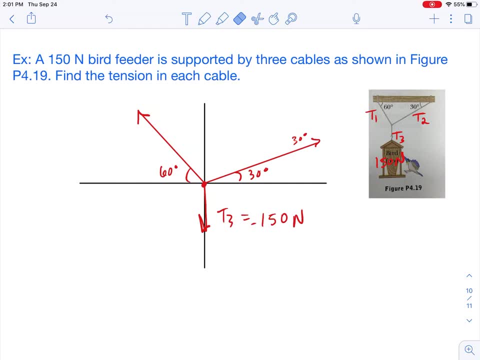 interior. that means that they are equal, So we can set that equal And that's going to just going to give us a little bit better idea Of kind of how to solve this problem. I kind of where to go, all right, and we have to use our knowledge of. 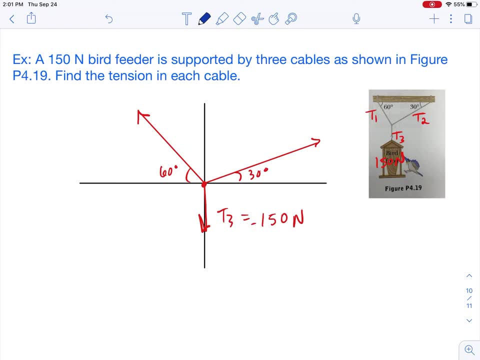 when we have an angled vector, we need to be able to break it into X and Y vectors, And so just trying to visualize here those X and Y vectors that we have to kind of utilize to our vectors When we have an angle vector, then we have to move those X and Y vectors forward. that's when we assume they are equal, or at least we have x and y vectors. that is, move their angle vector through our Bangladeshi victor and Susan peril And they. but that, and theussen, you'll need to start calling those x and y vectors. Thousle yourself. 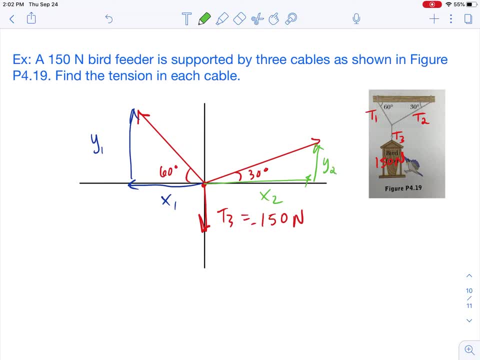 You know, just trying to visualize the new one you'll ada to when we do it to the new one, you'll Amen well that you would know that these Produkt will keep in us Which question kind of utilize to our advantage and use that those trig functions to help us with that. 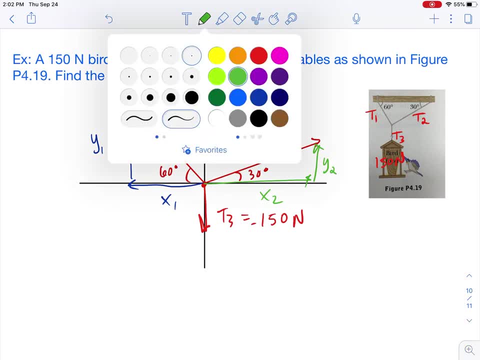 all right, in addition to Newton's laws. so the next thing that we're going to do, essentially, is we're going to solve for, like, what's the total y component and then what's the total x component, all right, and so if I were to solve for my total y component? 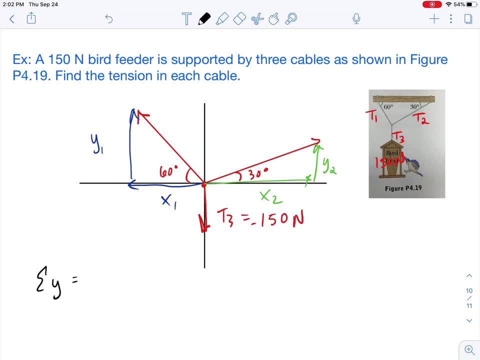 that's going to be my y1 plus my y2 minus my what would be t3. t3 is completely vertical, so that's like just the y component, and so how would we solve for y1, right? so here I have my 60 degree angle, so if I'm trying to find the hypotenuse in this case, which is t1, so why don't we just 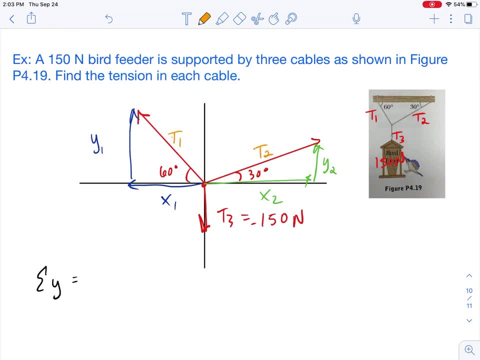 label that. so this is my y1 and then I'm going to solve for my y1 and then I'm going to solve: is T1 and this hypotenuse would be T2.. I'm going to go opposite and hypotenuse, So that's going to. 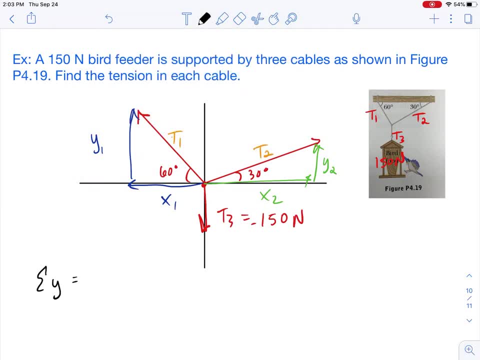 give me my sine trig function. So we're going to go T1 times the sine of 60, plus I got to do the same thing for T2.. So it's the same thing. I'm going to go opposite hypotenuse, So that's sine. 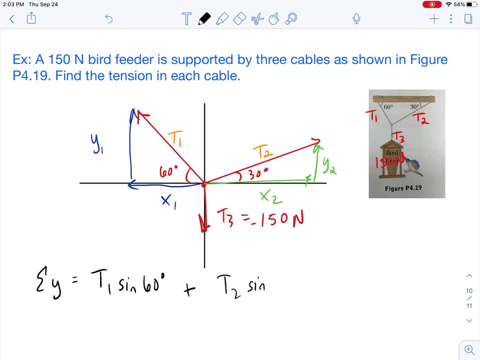 So that's going to be T2 sine of 30.. And then we're going to subtract the bottom Y component, 150.. And all of that should equal out to zero, Because there's no acceleration. everything is in equilibrium here, So everything's going to equal zero. 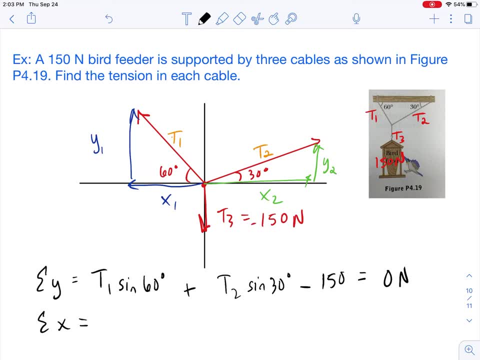 Now we're going to do the same thing for the X component. So I've got pretty much X1 and X2 are going to have to cancel out. and so how do we solve for x1? well, x1 is, if you notice, is going to the left. so 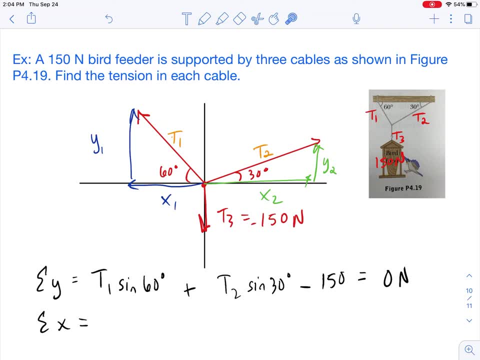 that's a negative component, all right. so, um, if i have t1 and x1, i'm going to use cosine, because cosine is adjacent and hypotenuse. so t, uh, so negative, t1 times the cosine of 60 plus. and the same thing on this side with a 30 x2 and t2, we're going to do um, t2 times the cosine. 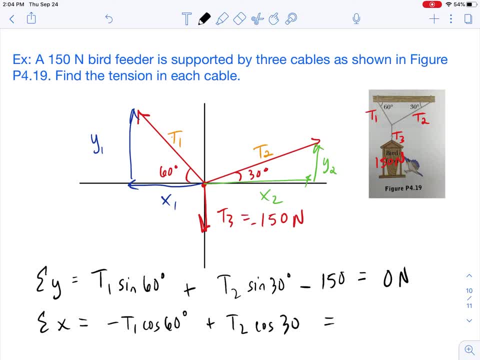 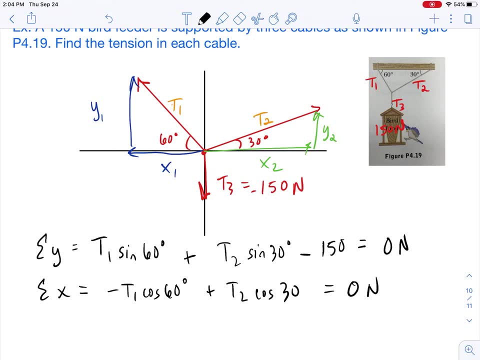 of 30, and that should also equal zero, all right. so now we have two equations and we have two unknowns, and so what we have to do at this point is we have to make a some sort of substitution, all right, where we can eliminate the two unknowns and make it just one. 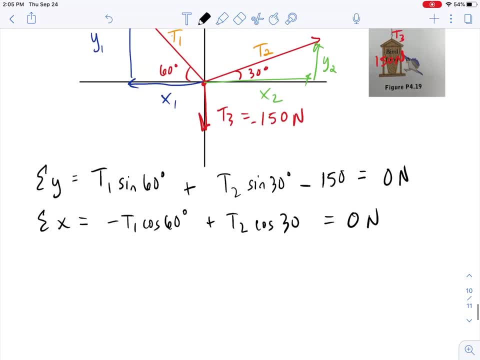 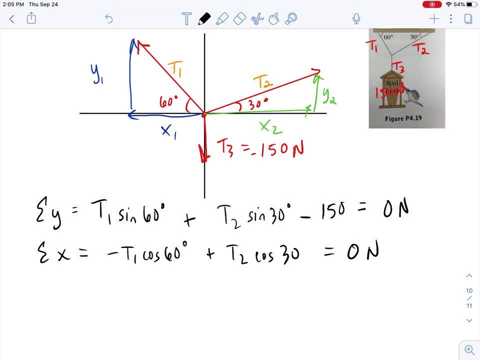 unknown. all right, and the way that we're going to do that is, we're going to use that. we're going to use this uh x total x component equation where we can swing this uh t1 across so we can add t1 cosine of 60 to this side. 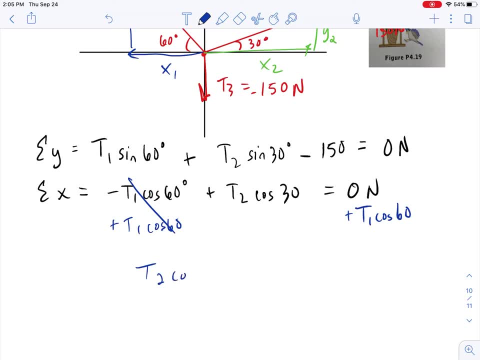 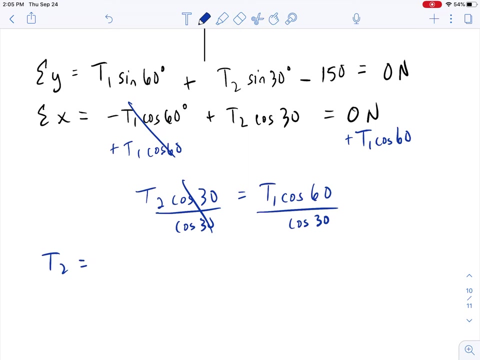 and so i'm just going to rewrite this: um, t2 cosine of 30 is going to equal t1 cosine of 60, and then i can get rid of this cosine of 30 to get t2 all by itself. so t2 equals t1 times the cosine of 60. 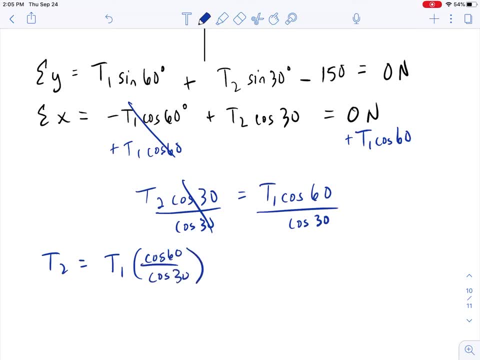 divided by the cosine of 30, and so we'll simplify this. so t2 equals t1 times 0.577. so now i've got, i've eliminated t2 into t1, and now what i can do is i can go back into the total y equation and make that substitution, and so that's what we're going to do at this point. 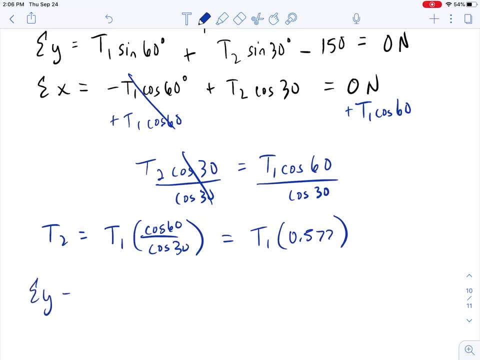 so if i go back to my total y equation, so t1 sine of 60 plus, and here, here's where i'm going to make that substitution, where i'm going to substitute this t1, 0.577 in for that t2. so it's going to look like this: um: 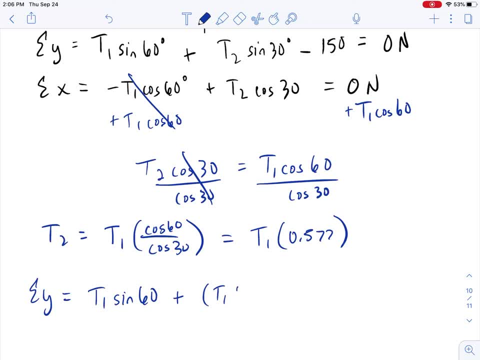 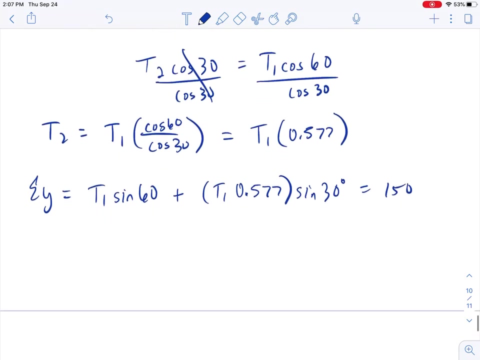 t1 times 0.577, times the sine of 30 degrees, and i'm going to just kind of swing this on the other side. so add 150, so that's going to equal 150. all right, now we're just a means of combining like terms. 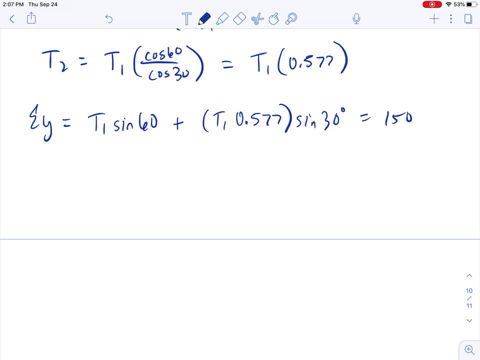 all right. so t1 um times sine of 60 gives us 0.577, gives me um t1. well, really, it gives me um. i should have rewrote the other other way, 0.866 t1 plus, and then we're going to do this here- 0.577 times the sine of 30.288. 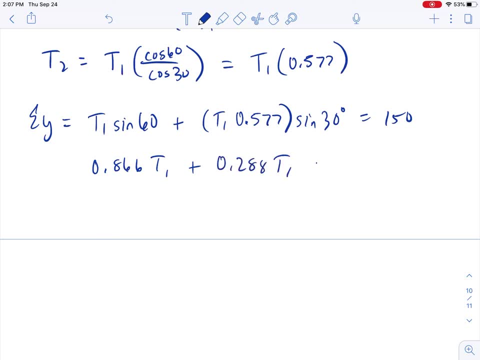 so this is 0.288. t1 equals 150.. so that's something that's bi-variable, right, okay? so immediately we're doing like this: here goes the number: this becomes our sine times, the sine of 30.288 times the sine of 30.288. 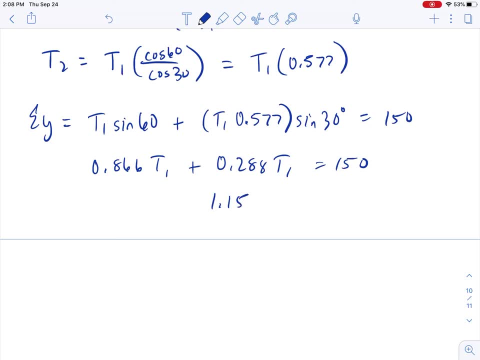 so our sine times 1.61: t1 squared according to this equation, and we will just call and then we will divide by 1.15, on both sides. also, we can use the square root of trains. so what? this is what. this is our so short years. one of your bills, and then we just add them up. so 0.866 plus 0.2, 80 gives me 1.15, to ese 가능ely equals 150, and then we will divide by 1.15 on both sides, so t1 comes out to be 130 newtons. so now we've solved the. 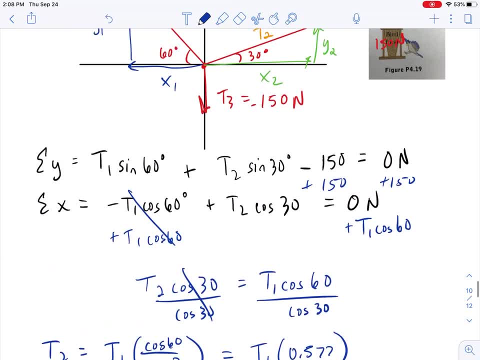 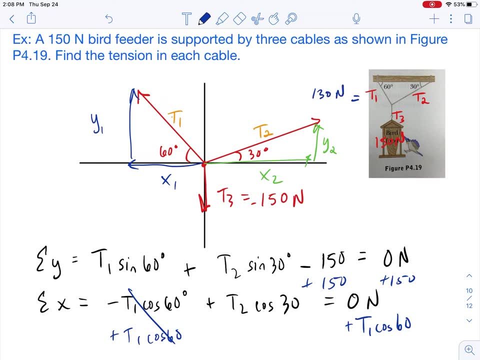 truth. so t1 comes out to be 130 newtons. so we're going to take over the brayle, sfeter and vocês t1. you know this is 130 newtons. now the only goal we have left is to solve for t2 and that. 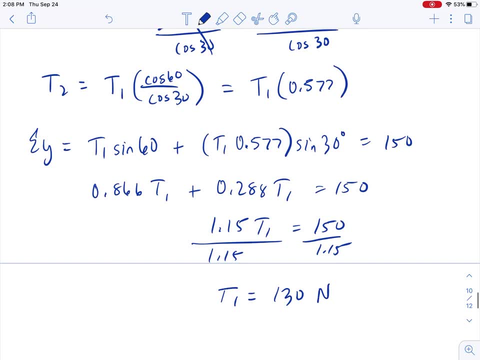 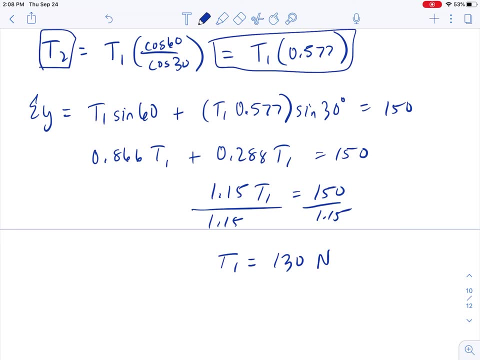 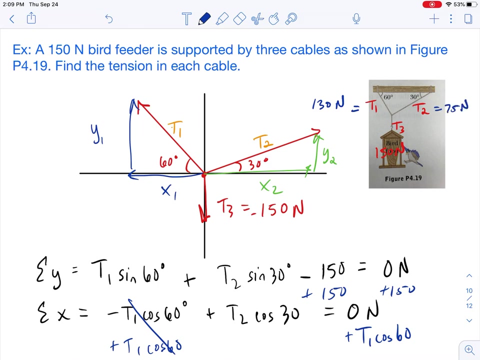 becomes really easy, because t2 equals t1 times 0.577. so t2 is going to equal t1, just 130 times 0.577, and we get our answer of 75 newtons. all right, and so now you know all of them. t1 is 130. 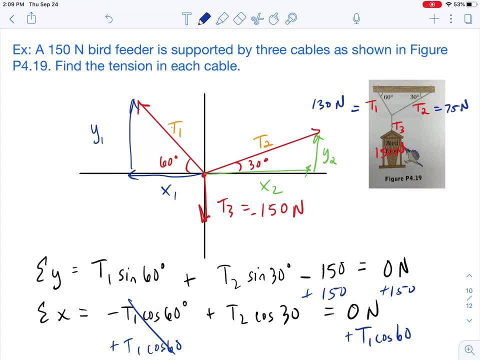 t2 is 75 and t3 is the 150, so I hope this video is helpful for you in solving your own tension problem, where the angles are not the same as always. like and subscribe if this video has helped you.